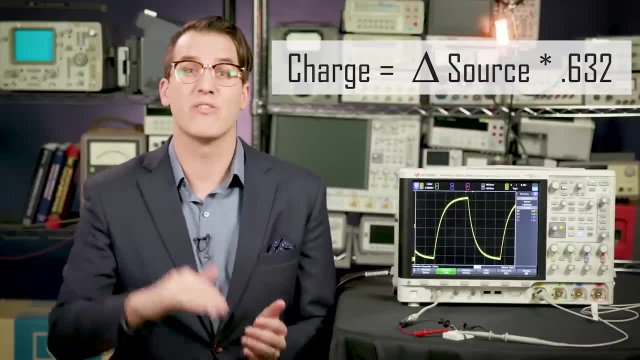 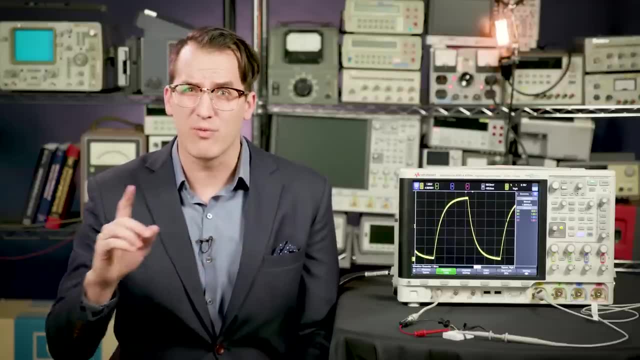 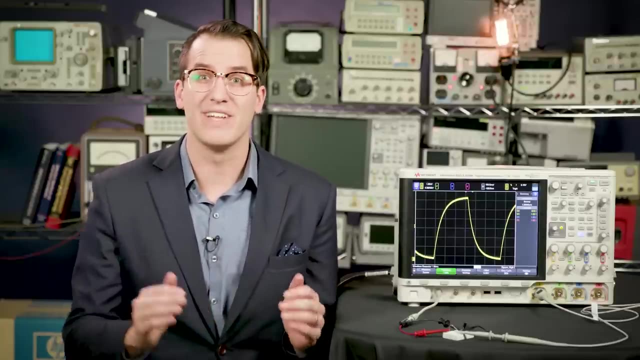 What this means is that a capacitor will charge up to 63.2% of the source delta after one time constant. From a settling perspective, if we wait a period of one time constant, we move 63.2% closer to our final value. After a second time constant, we move another 63.2%. Essentially, it 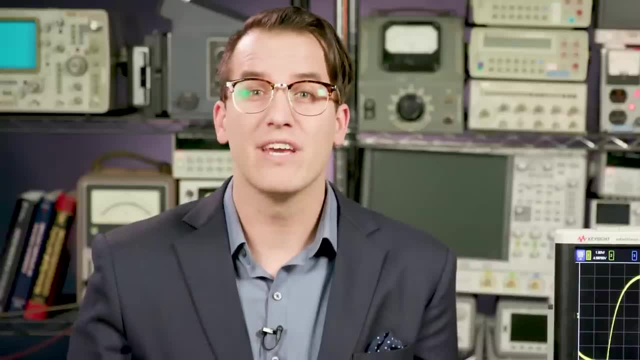 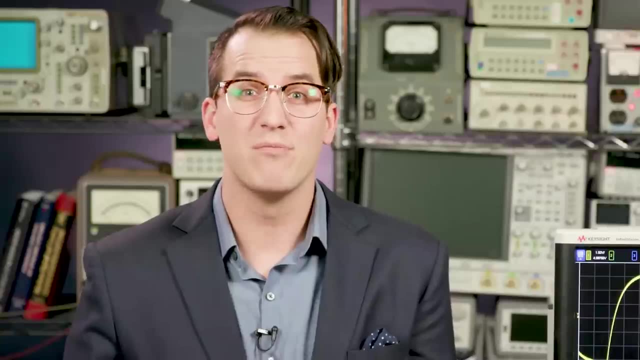 drops to 36.8% of its starting value. Now think about this For the period of the second time constant. we're basically dealing with a new delta source value. So instead of moving from 10 volts to 0 volts, you're now moving from 3.68 volts to 0 volts. So after the second time, 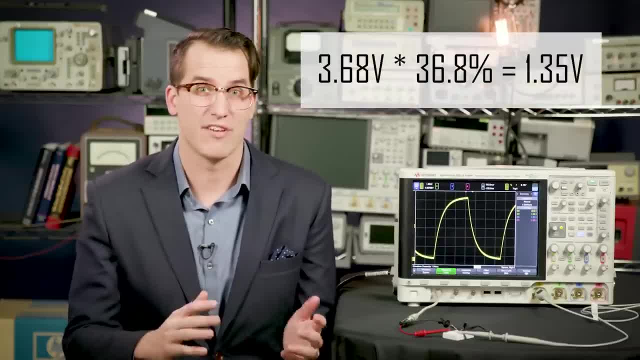 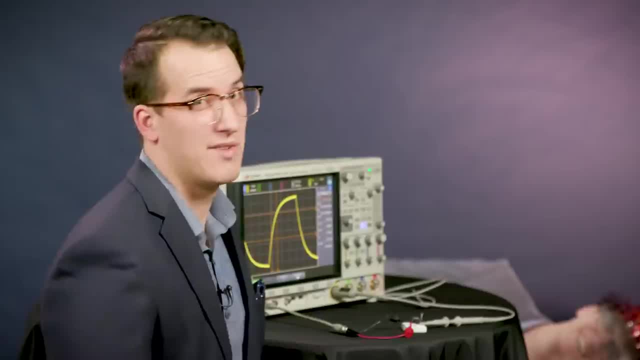 constant you'll end up at 3.68 volts times 36.8%, roughly 1.35 volts. After five time constants you'll be 99% of the way to your final voltage. After five time constants. people generally. 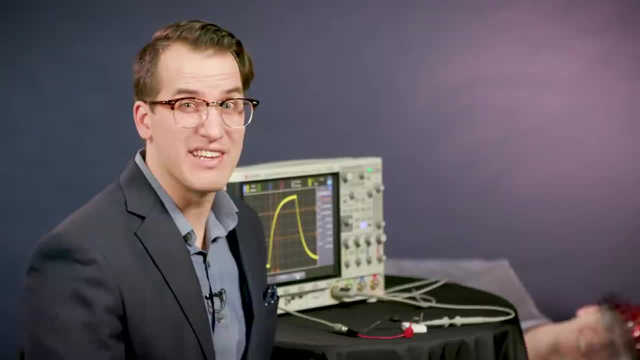 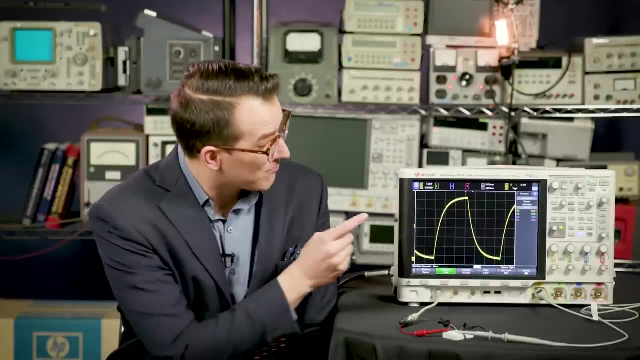 agree that for all practical purposes, the signal has settled and the inductor or capacitor is fully charged or discharged. So if you were to plot this out, your signal will look like an exponential curve. This is where the oscilloscope comes in For this simple RC circuit with a square wave. 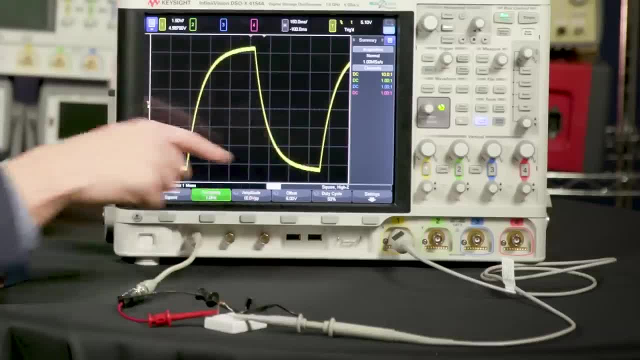 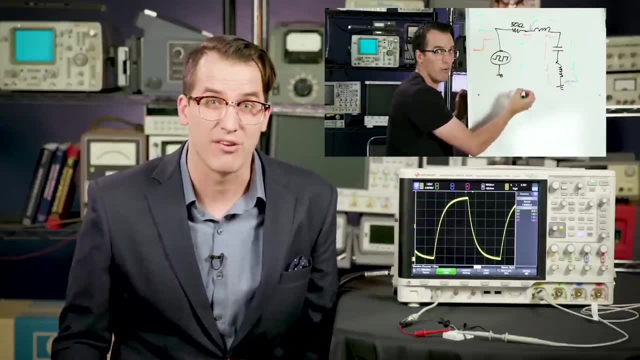 input we see an exponential curve both up and down. For more on step response, check out the parasitic inductance and AC step responses video which I'll link to in about a minute 30. But you'll probably want to see this first. To measure the time constant with an oscilloscope, I'm going to 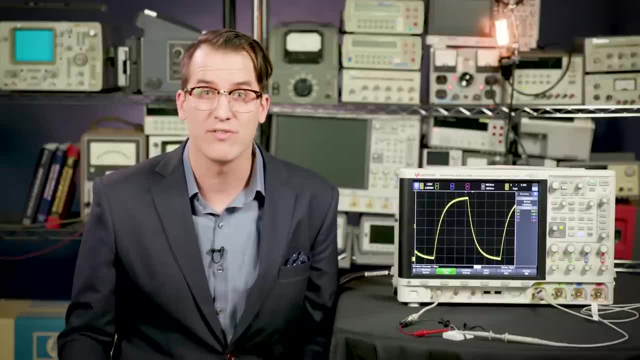 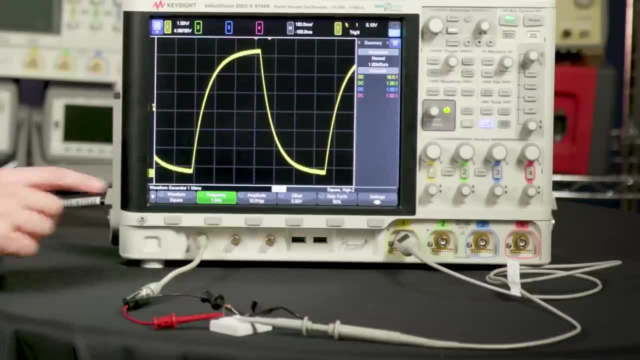 simply pick two reference points on the decaying or growing portion of your signal and see how long it takes to decay or grow: 63.2%. Here's our simple RC circuit being supplied with a square wave from my function generator going between 0 and 10 volts For measuring the time. 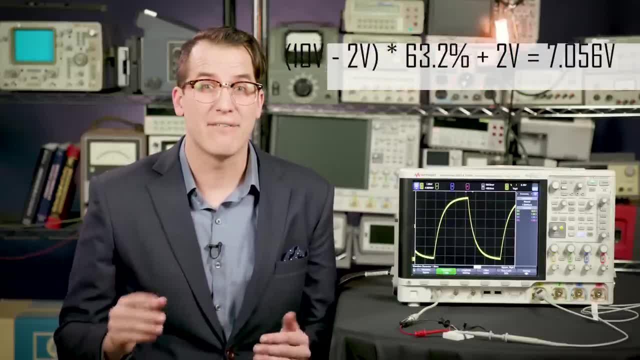 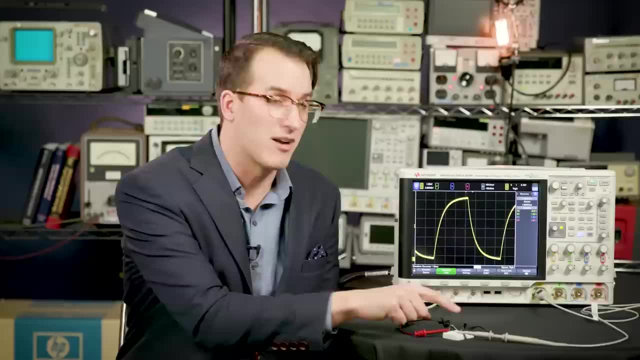 constant. let's pick 2 volts as a starting point, which means that after one time constant, we should end up right at 7.056 volts. We're probing the voltage across our capacitor, so it should be easy to measure the time constant. So let's turn on Curve. 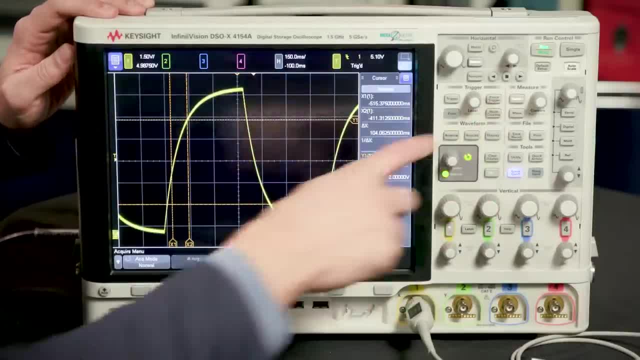 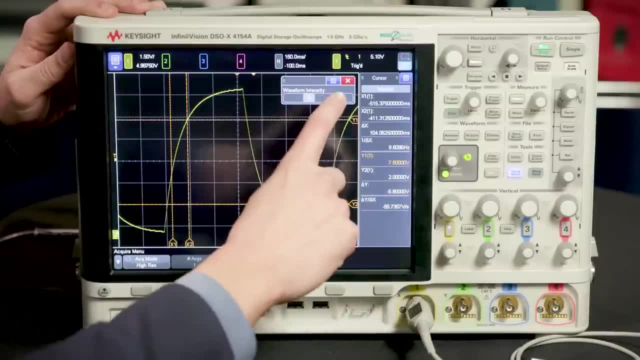 and to get a cleaner acquisition, let's go into Acquire and turn on High Resolution mode And then it's a one hertz signal, so it's going to be a little slow updating. And let's bump the waveform intensity all the way up to 100 so we can see it. Let's put our Y1 cursor at our starting. 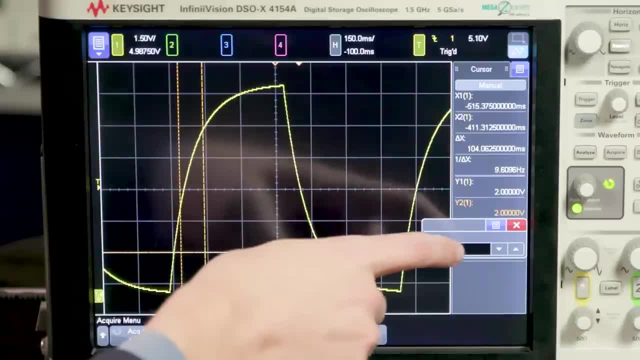 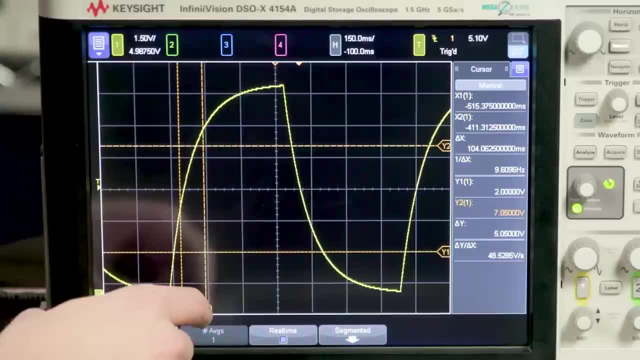 voltage, which is 2 volts, and our Y2 cursor at 7 volts, 7.056 volts, our calculated value. And now we're going to move the X cursors to line up with the intersection of the waveform and the Y cursors. We're going to do the same with both. 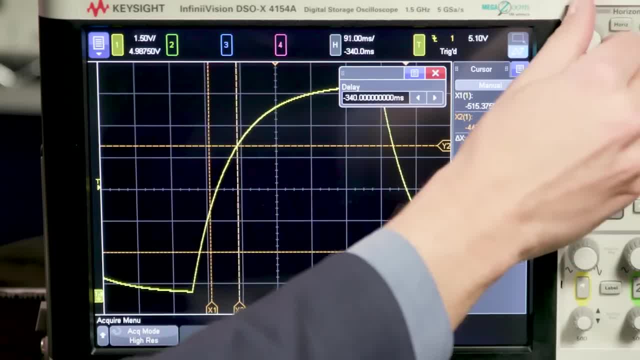 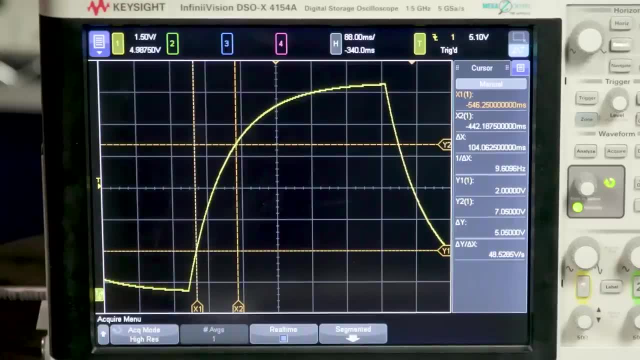 Let's zoom in a little bit here just to get some better horizontal accuracy out of our measurements. here I'm going to move the X1 cursor right there And this distance between our X cursors is our time constant, So that value that we're measuring. 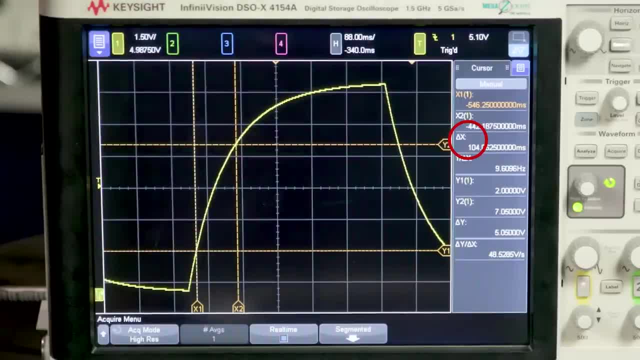 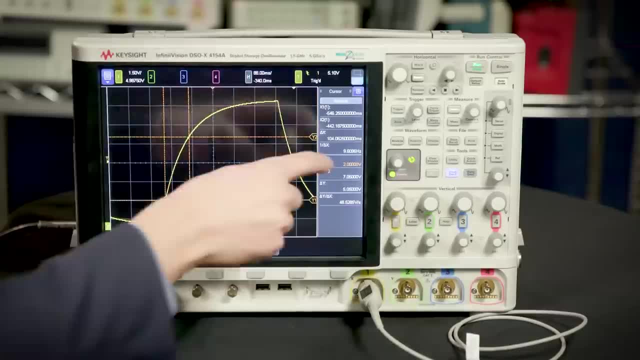 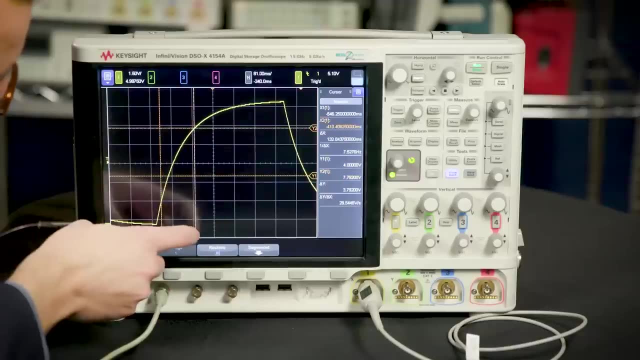 is 104 milliseconds. So we can say that for this circuit our time constant is 104 milliseconds. To prove the time constant is actually constant, let's do it again, but starting from 4 volts, So we can see again: we're measuring right around 104 milliseconds For a more robust time constant, 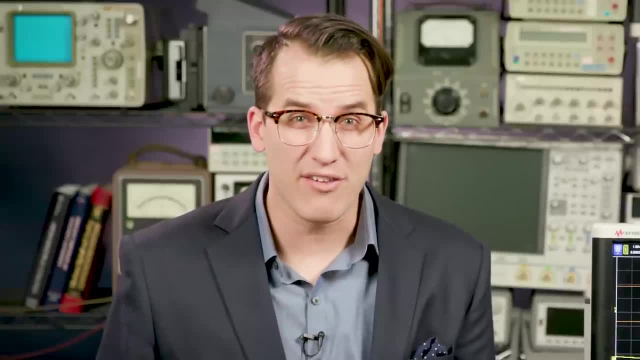 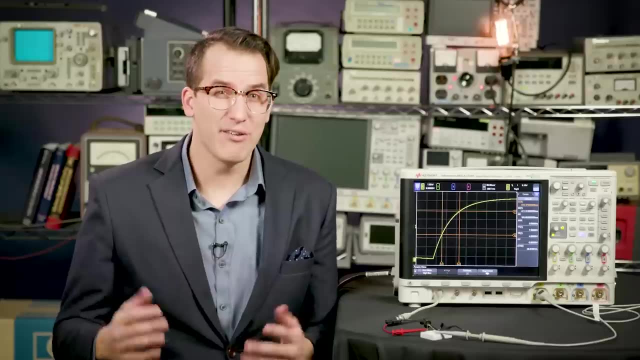 measurement. do this a few times with a few different captures and add a few different start or stop voltages and take the average. I'd also recommend staying towards the middle of the decay, as it's possible to get some non-linear effects right at the beginning. 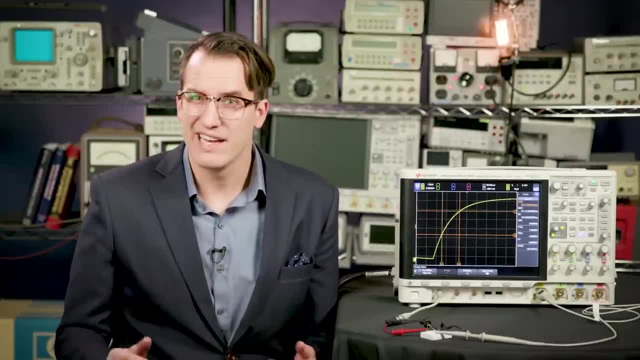 An example of this is the parasitic inductance video linked above and in the video description. So we're going to take a look at some of the parameters that we're going to use. We're going to take a look at some of the parameters that we're going to use. So we're going to take a look at some of the parameters that we're going to use. 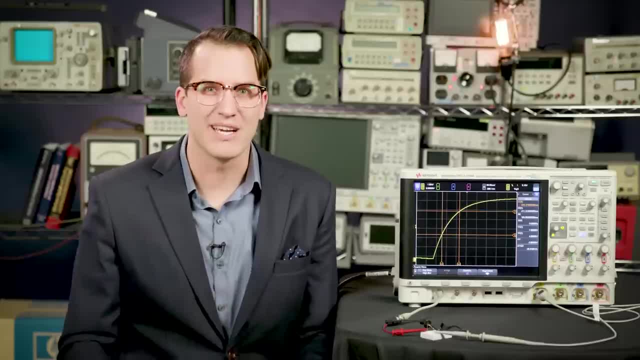 So we're going to take a look at some of the parameters that we're going to use. We're going to take a look at some of the parameters that we're going to use. So, now that we have a good idea of what our time constant is, we can compare it to our 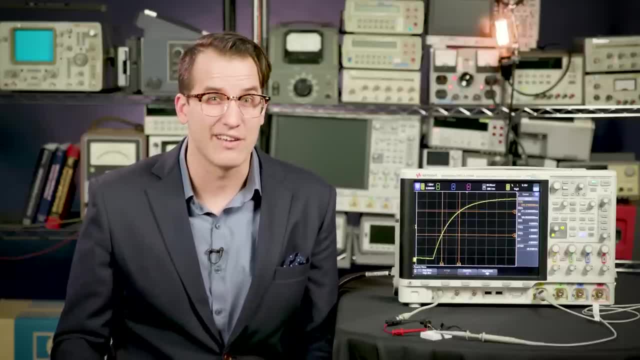 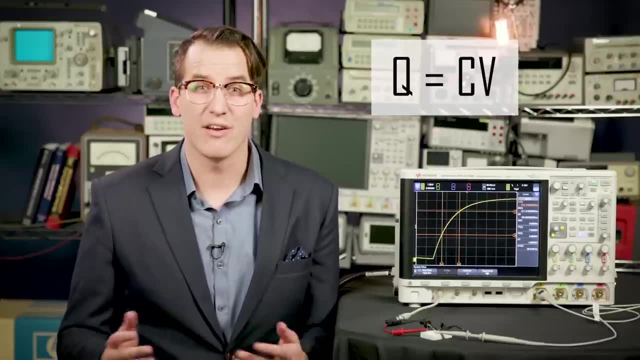 calculated value. Before you do that, we should probably learn how to calculate the time constant Without going through the math. you can do some fancy substitutions using the formula for charge, Q equals CV and Kirchhoff's law, and you end up with the elegantly simple tau equals R times C. 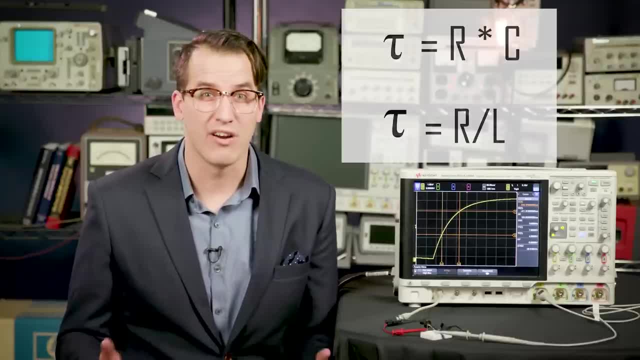 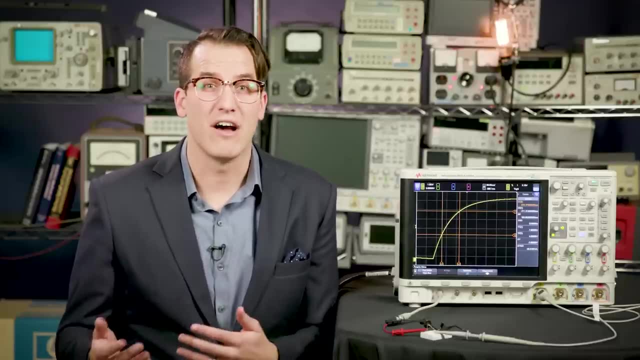 for an RC circuit and tau equals R divided by L for an RL circuit. For this circuit we're using a 1 kilo ohm resistor and a 100 microfarad capacitor, so our calculated value is 100 milliseconds, which is pretty darn close to our measured value, Just for kicks. 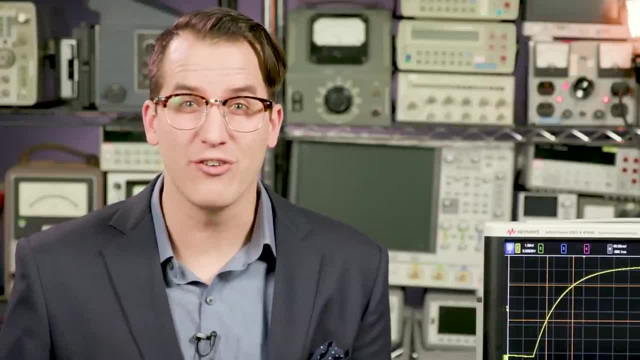 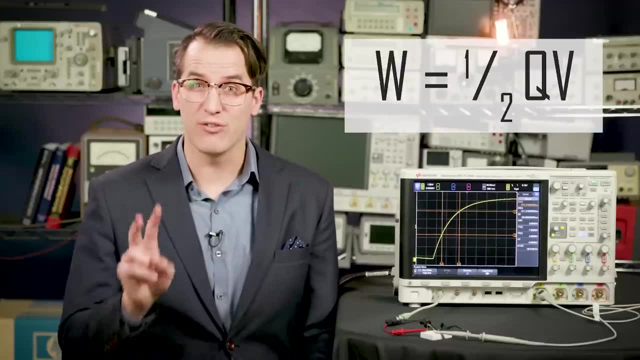 let's go a little deeper. After one time constant, we know that the charge on the capacitor will be 638 microcoulombs. using Q equals CV and the energy stored in the capacitor will be roughly two millijoules based on W equals one half QV. If at some point, this resistor load were to be 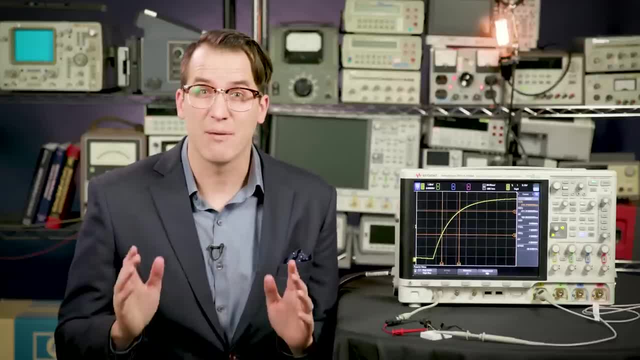 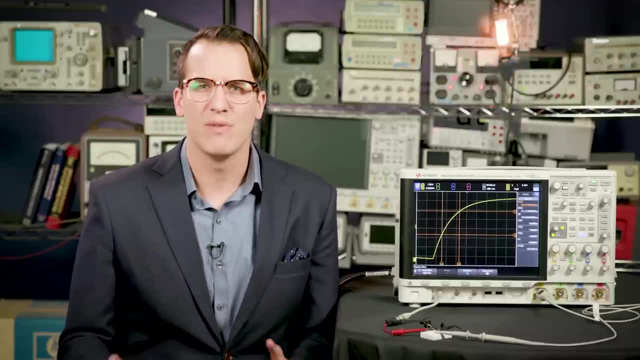 removed after one time constant or there's a switch opening up the capacitor or inductor will throw all of that stored energy back at your source. If you aren't careful, that can cause serious damage. Remember, inductors resist a change in current, so if you open a switch, that 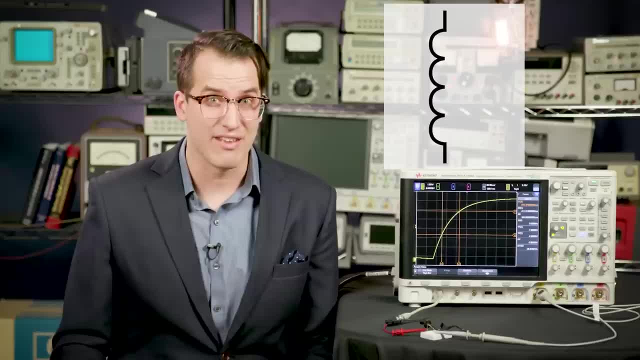 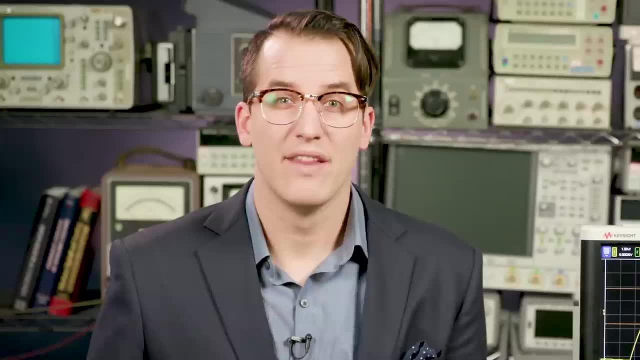 is providing current to an inductor. the inductor is not going to allow that instantaneous current change. To protect against this, you can put a diode in parallel with the inductor to allow it to discharge. This is called a freewheeling or flyback diode. You can also build an RC. 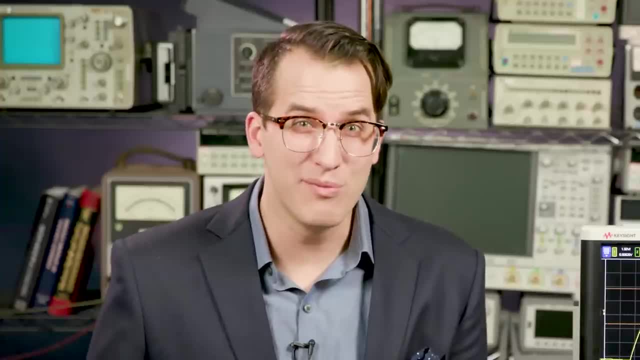 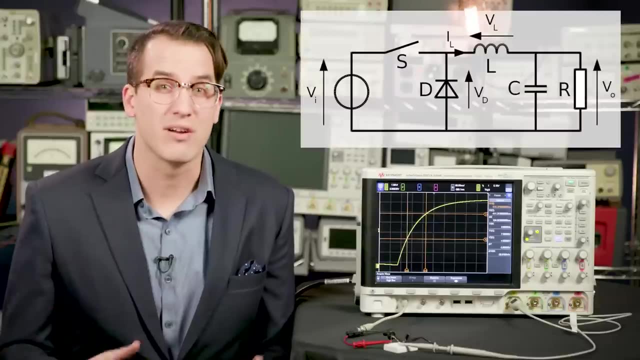 snubber if you need a faster current decay. It's not all doom and gloom, though. The charge storage can be quite useful. It's actually the fundamental theory behind switch mode power supplies. Take a buck converter, for example, which is used to efficiently step down voltage. 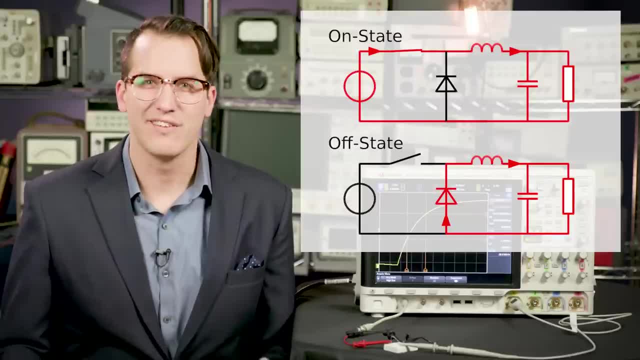 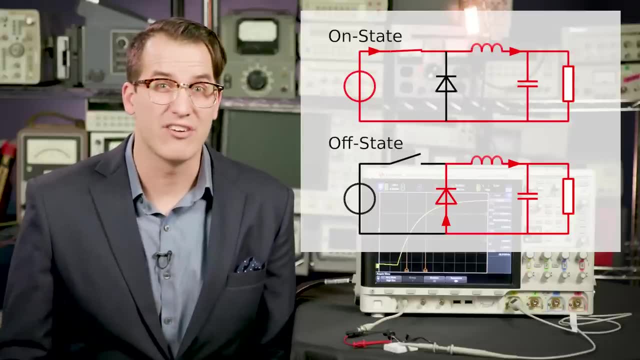 When the switching transistor is closed, the on state- the inductor is charging up, and when the switch is open, the off state the inductor is actually powering the load. The capacitor here generally acts as a filter capacitor to help remove some of the inherent. 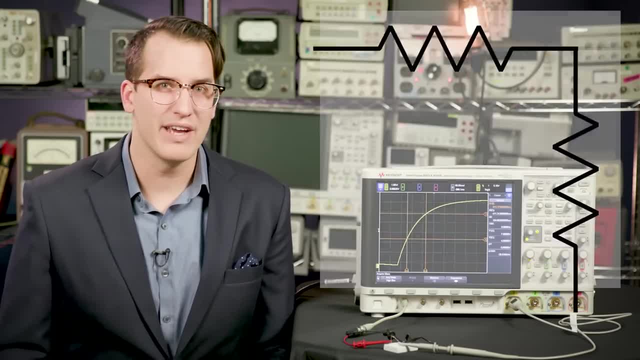 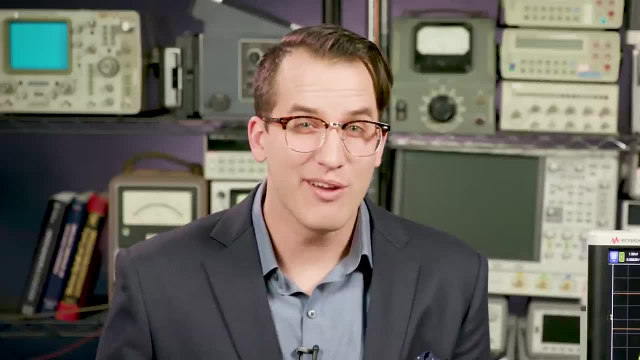 ripple in this type of design. This is useful because, unlike a resistive voltage divider which also steps down voltage, you don't lose half your energy in that other resistor. You could also go old school and use RC and RL circuits in conjunction with a comparator to form an